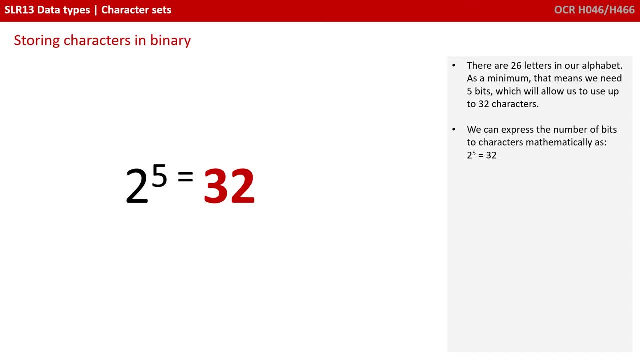 We can express the number of bits to characters mathematically. for example, 2 to the power of 5 equals 32.. That's because binary is base 2,. there are two possibilities for each, for example, with five bits- 0 or 1, and to the power of five, because there are five bits. 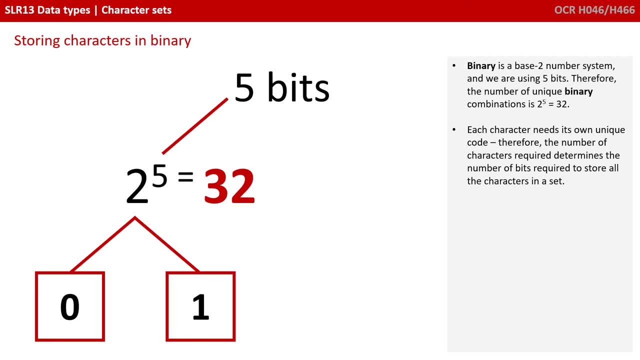 You sign dice, then add the fastCode and enter the character value 5, and the net value of the next character, luxurious account. This means that the number of unique binary combinations for 5 bits is 32.. Each character must have its own unique code. 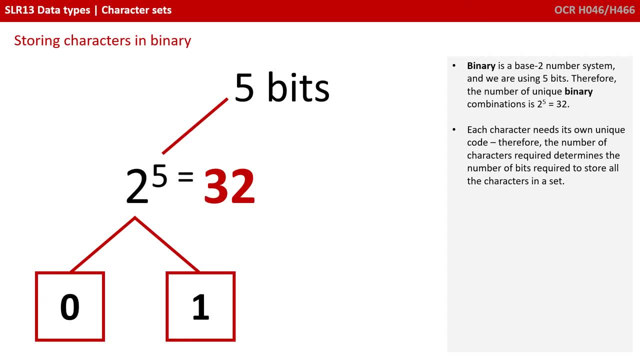 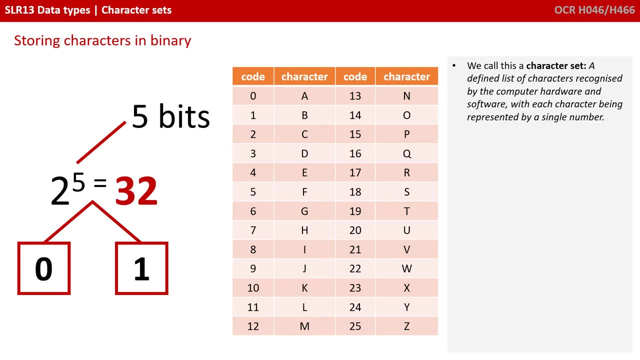 which determines the number ofufen key, which means that each character must need all five or multiple numbers to need the number ofobjects to store the characters in a set. We call this a character set, a defined list of characters, a defined list of characters in our language and classified by Text. Howів. 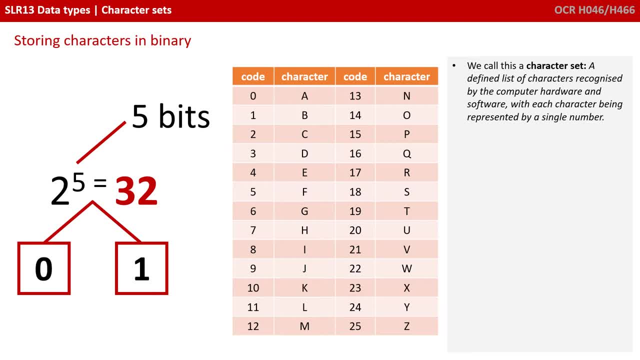 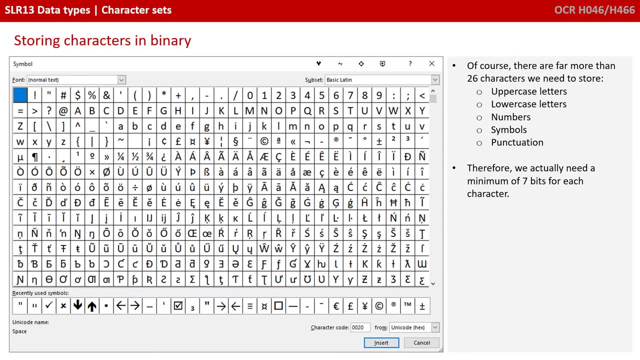 All of verse count three characters inそれ, one by oneThis means we can set different characters in the sequence recognised by the computer hardware and software, and each character represented by a number. Of course, there are more than 26 characters we want to be able to store. 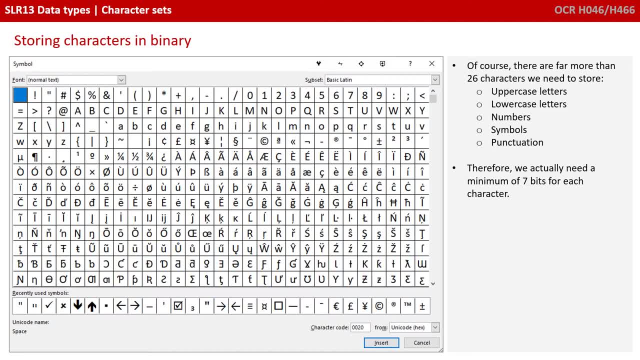 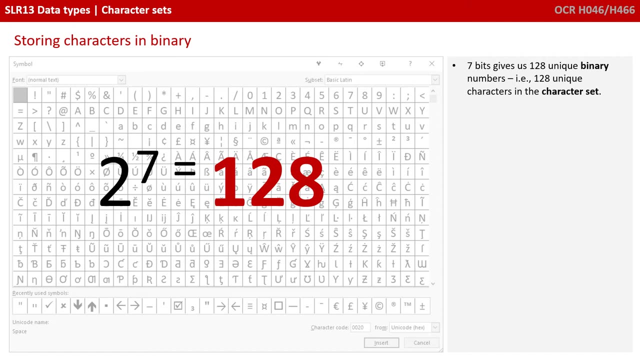 There are both upper and lowercase letters, and that doubles the number of characters we need instantly. But there's also symbols such as pound signs, brackets and punctuations. Therefore, we actually need a minimum of 7 bits for each character, That is, 128 unique binary numbers, 128 unique characters in the character set. 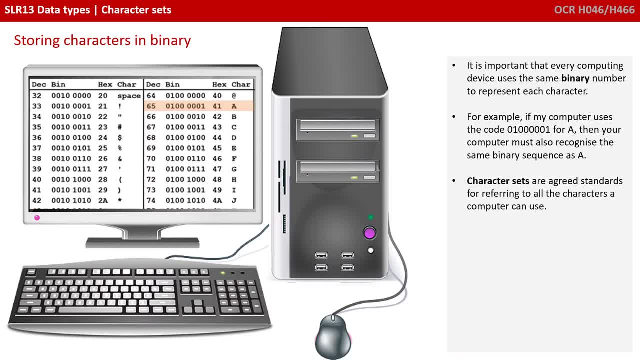 It is important that every computer is using the same binary number to represent each character. For example, if my computer uses the code 0, 1, 0, 0, 0, 0, 0, 0, 1 to represent the capital letter A. 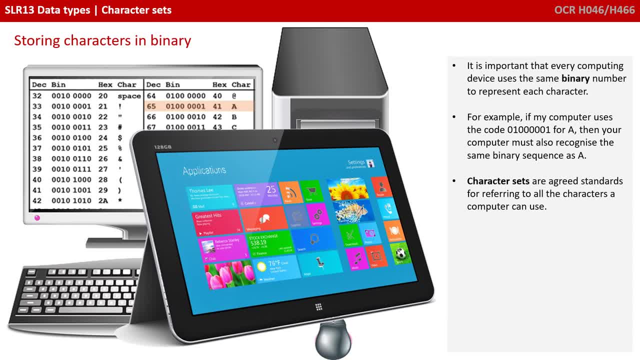 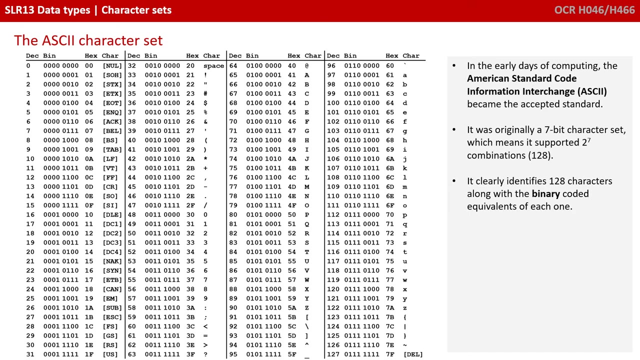 then your computer must also recognise that same binary sequence as a capital letter A also. Therefore, character sets are agreed standards, an agreed way of numbering all the characters that computers use. In the early days of computer science, ASCII, or the American Standard Code for Information Interchange, became an accepted standard. 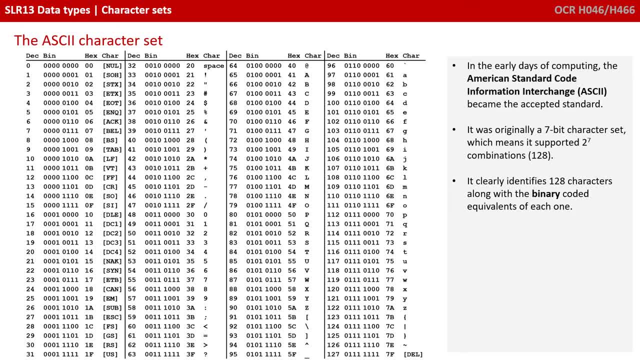 ASCII were a 7-bit character set. This means there were 2 to the power of 7 combinations of bits, which is 128 different combinations, and therefore it identified 128 characters and their binary codes or binary equivalents. This was extended to an 8-bit character set. 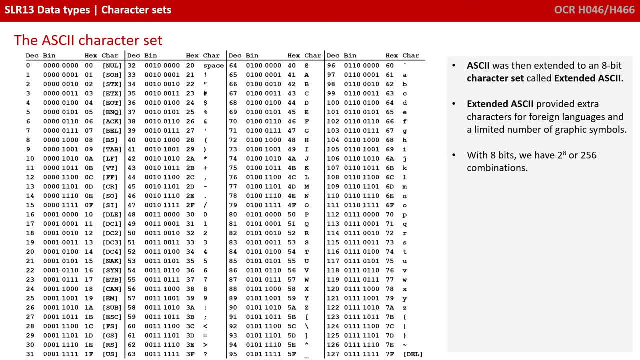 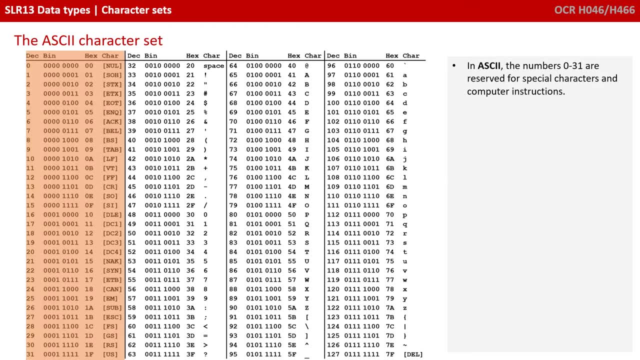 called Extended ASCII, which provided for characters from some foreign languages and other useful graphical symbols. In 8 bits we have 2 to the power of 8 combinations and therefore 256 characters In ASCII. the numbers 0 to 31 were reserved for special characters and instructions to the computer. 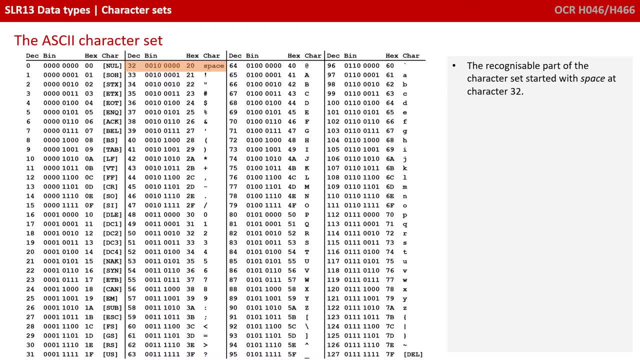 So the recognisable part of the character set started with a space at number 32.. Purely out of interest, character 7 caused your computer to beep. This was before the days of sound cards, And character 13 was a new line character. 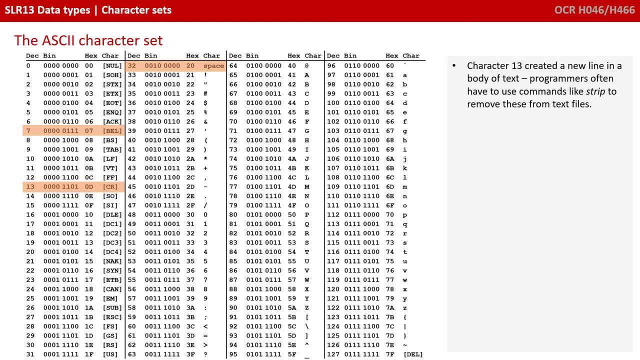 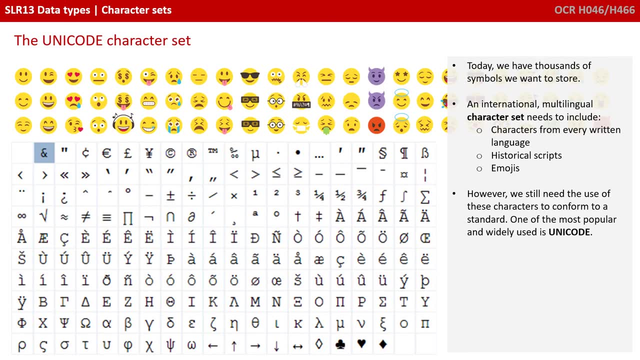 which is why you often have to use commands like STRIP in programming when reading data from files to remove or strip these from the ends of lines and text. Today we have thousands of symbols we want to be able to store. We want a fully international and multilingual character set. 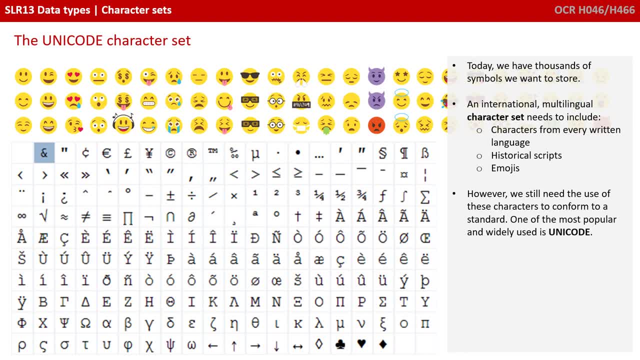 which includes all the characters from every written language, historical scripts, plus more modern characters such as emojis. These need to also conform to a standard, and this standard is known as Unicode. Unicode is implemented in slightly different ways for different purposes. For example, web pages may use a variant known as UTF-8,. 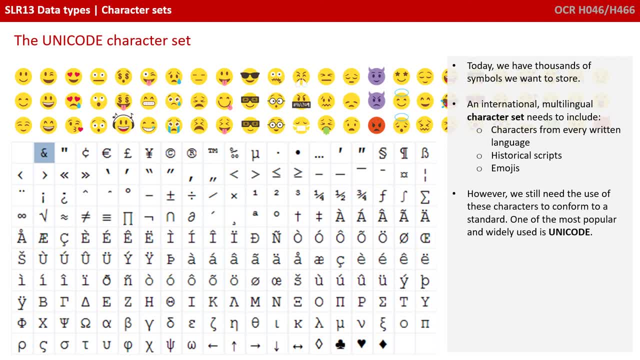 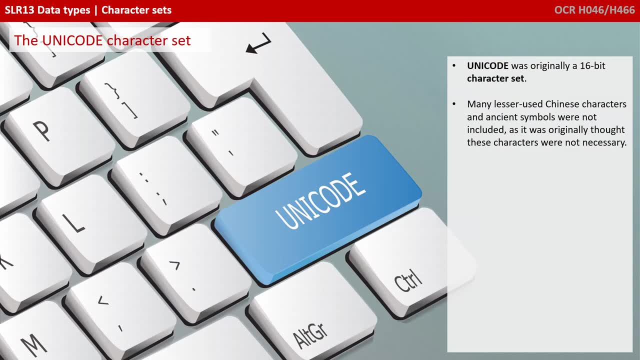 where the first 8 bits are the same as ASCII and the other characters are encoded with 32 bits. Unicode was originally a 16-bit character set. Many lesser-used Chinese characters and ancient symbols were never used. Many lesser-used Chinese characters and ancient symbols were never used.